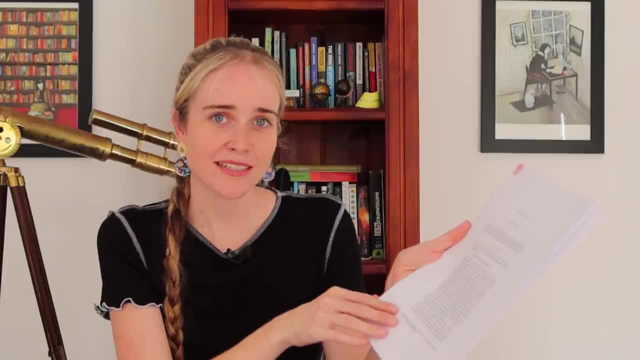 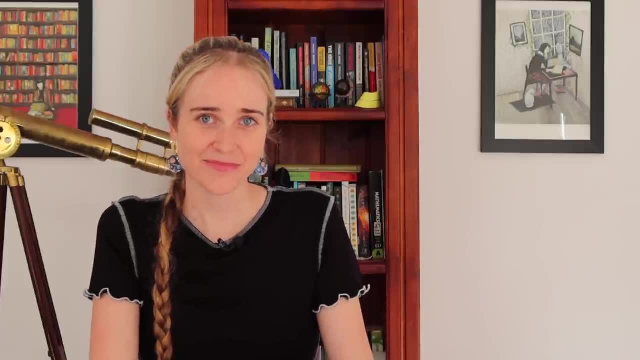 of mathematically gifted children. This report is Clements's thoughts and findings on Tao, including the results of a math test given to him. So let's take a look at it. It was the day before Terence's eighth birthday, the 16th of July 1983.. 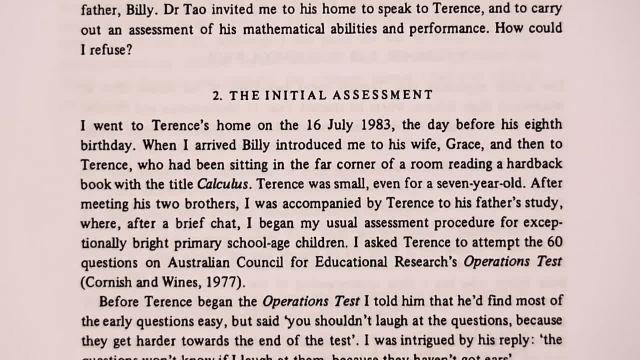 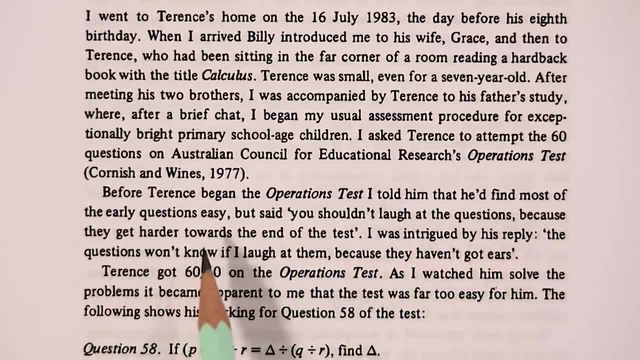 Exactly 38 years ago and it says here that Terence was given an operations test Knowing that he might find the first few questions too easy. Clements says you shouldn't laugh at the questions because they get harder towards the end of the test. And Terence has an interesting reply. He says: 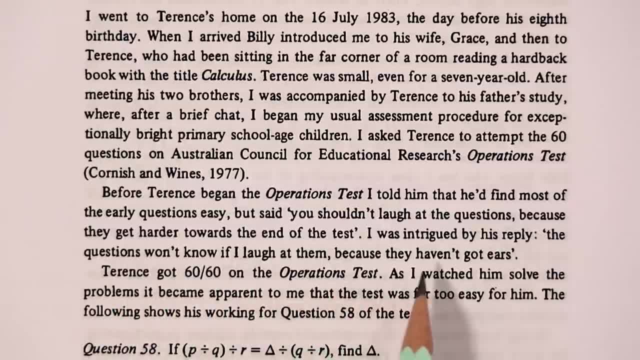 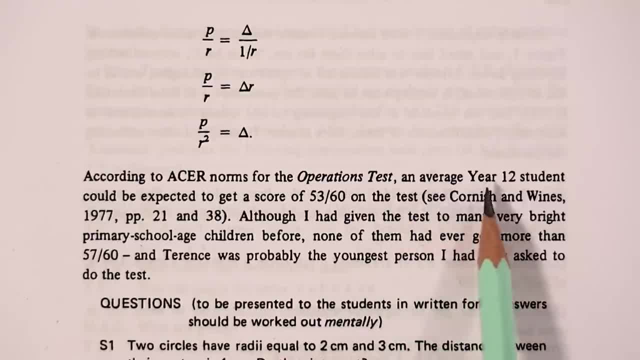 the questions won't know if I laugh at them because they haven't got ears. He went on to score a 60 out of 60 on this test. On average, a year 12 student taking the same test would be expected to get a score. 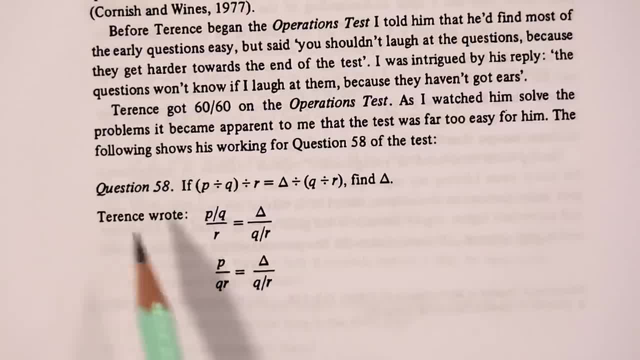 of only 53 out of 60.. And here's one of those example questions. Question 58 asked if p divided by q, divided by r, is equal to delta divided by q divided by r, then find delta. And here is seven year old Terence's answer. He writes it out as a fraction and then just does a bit of algebra to rearrange for delta. 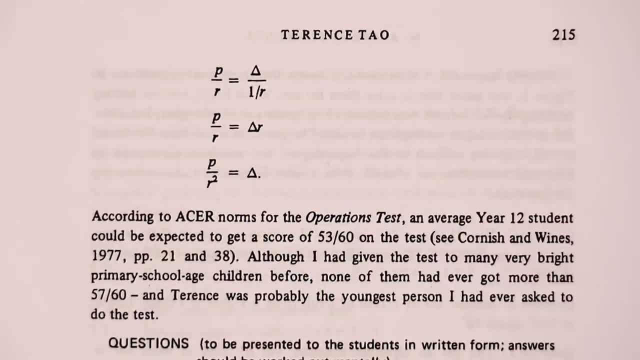 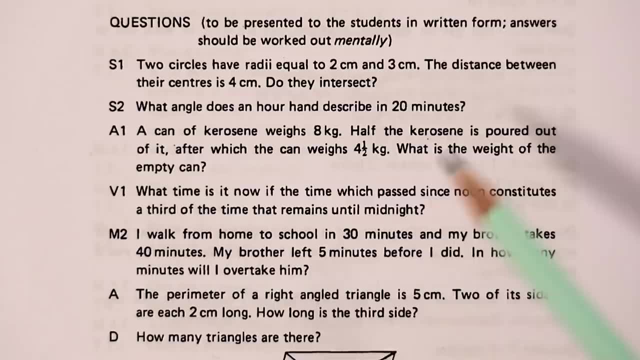 Getting it to be p over r squared. Although it was clear to Clements that this test was too easy for Terence and they'd need to move on to some more difficult things, This next set of questions were presented to him and they had to be worked out mentally. They include things like: what angle? 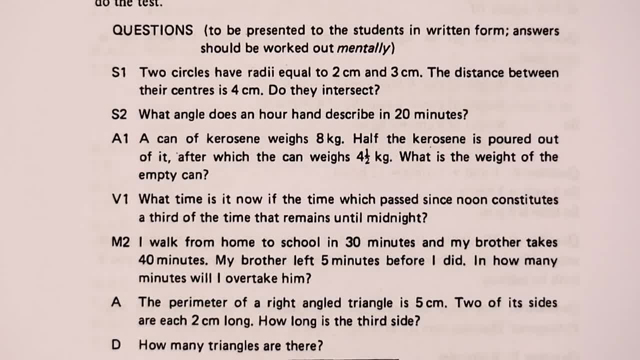 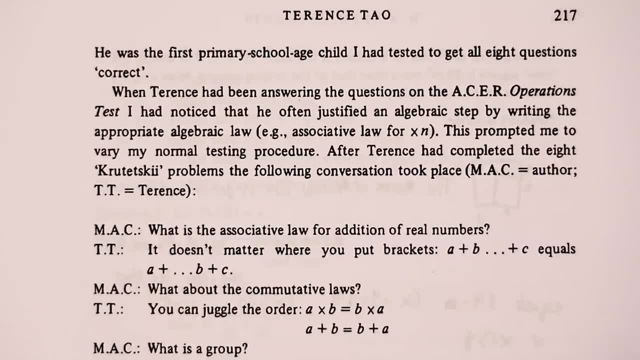 does an hour hand describe in 20 minutes Terence got all eight of these questions correct as well in a total time of nine minutes. Clements noticed that while Terence had been solving the questions, he often justified an algebraic step by writing the appropriate algebraic law, For example the associative law next to it, And so that prompted. 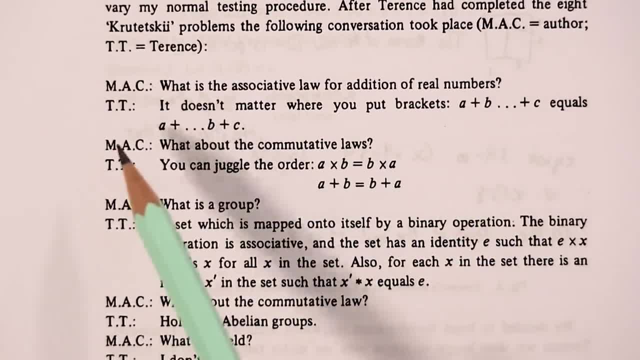 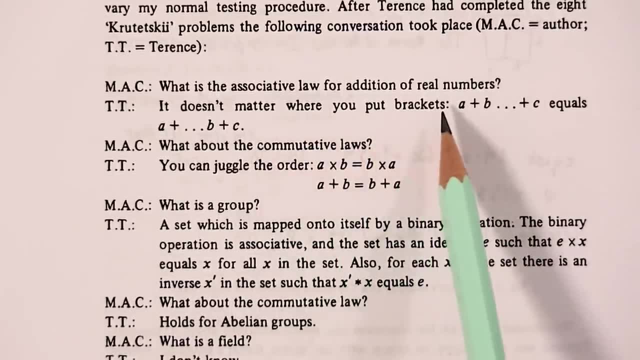 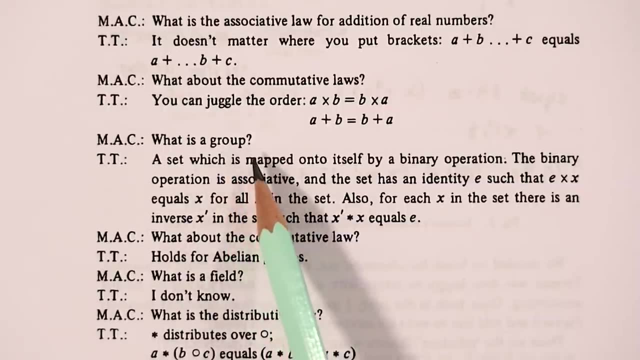 this following very interesting conversation. Clements asked What is the associative law for addition of real numbers. Terence answers that it doesn't matter where you put the brackets. He also gives a correct definition of the commutative laws And he also gives a correct definition of a group. 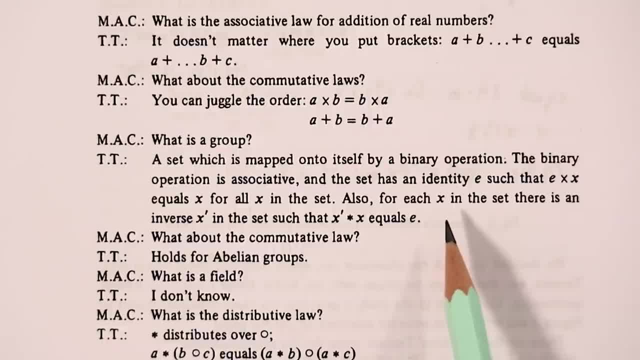 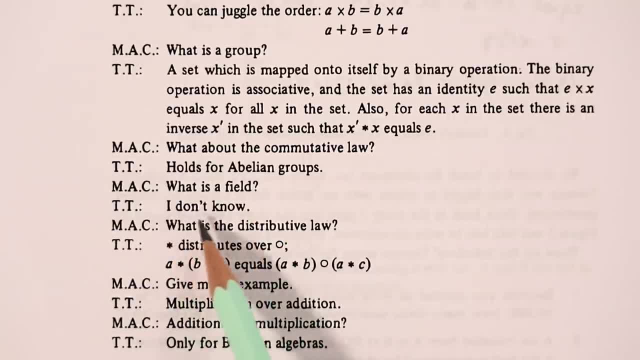 something that most math students don't encounter until university. However, it seems that the first thing to stump him was being asked: what is a field? Terence replies: I don't know, Given that I barely have a grasp on what a field is. now, I think it's forgivable, for 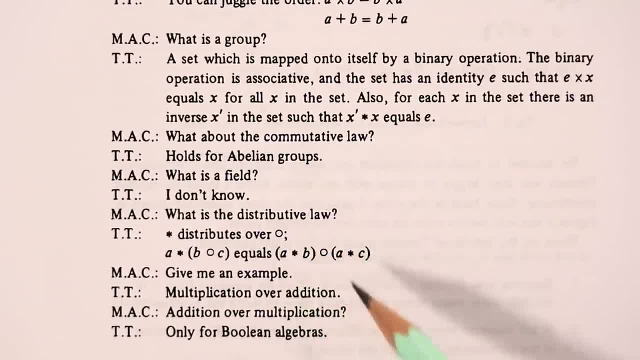 seven year old Terence not to know that either. He does, however, know about the distributive law and gives the example multiplication over addition. Clements asks if addition over multiplication is an example, but Terence replies only for Boolean algebras. 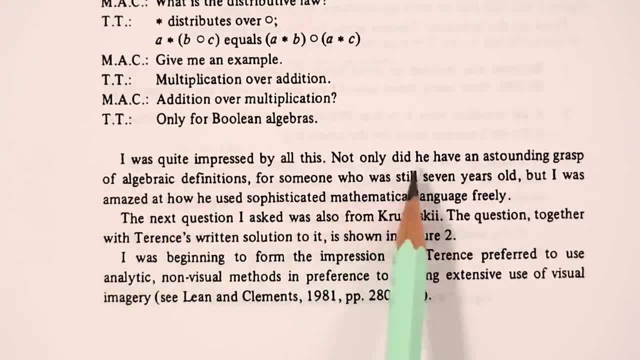 Clements was quite impressed by all of this. Not only did he have an astounding grasp of algebraic definitions for someone who was still seven years old, but I was amazed at how he used sophisticated mathematical language freely. I was beginning to form the impression that Terence preferred to use analytic non-visual. 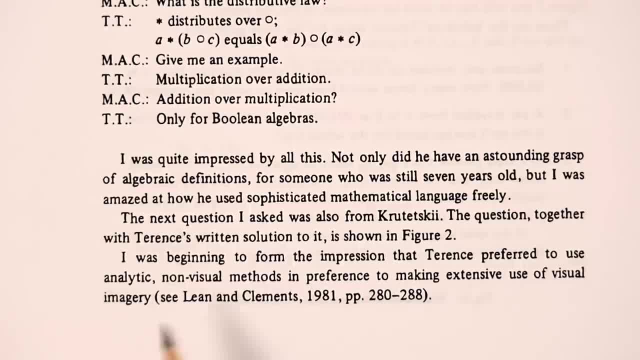 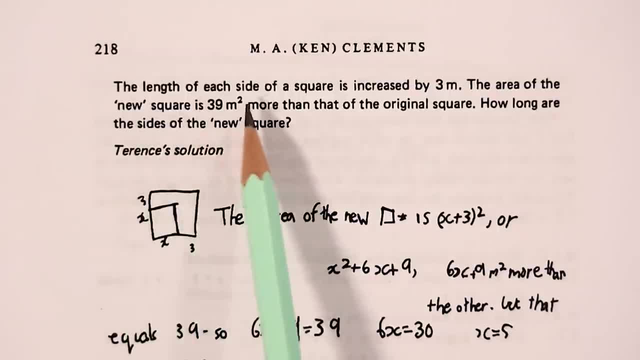 methods In preference to making extensive use of visual imagery. Here's one of Terence's actual written solutions to a question that says the length of each side of a square is increased by three meters. The area of the new square is 39 meters squared more than that of the original square. 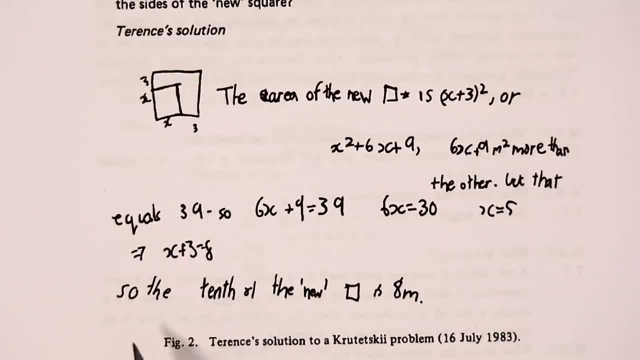 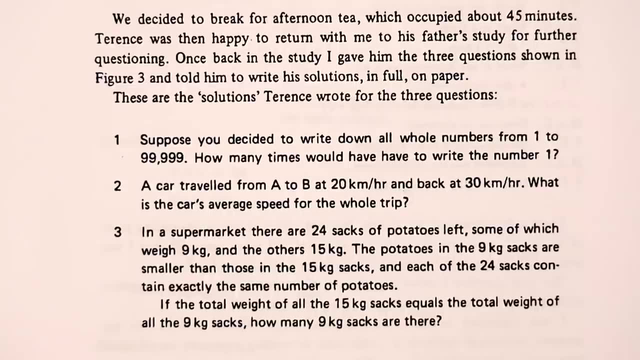 How long are the sides of the new square? Terence correctly finds that the length of the new square is eight meters. The next set of questions given to Terence include: suppose you decided to write down all the numbers from one to 99,999, how many times would you have to write the number one? 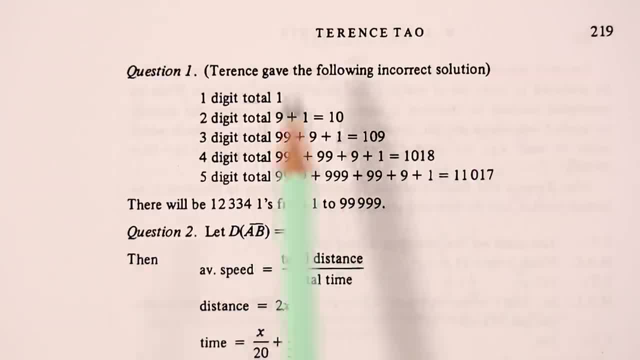 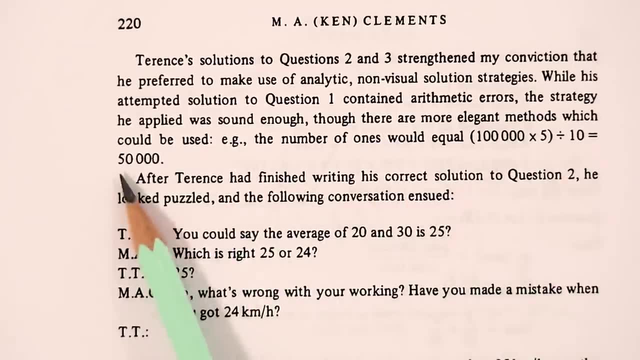 This one Terence actually gave an incorrect solution to, although still an answer that shows plenty of critical thought about the question. Apparently, the correct solution here is 50,000.. He struggled a little bit with a few more of these questions And Clements says: 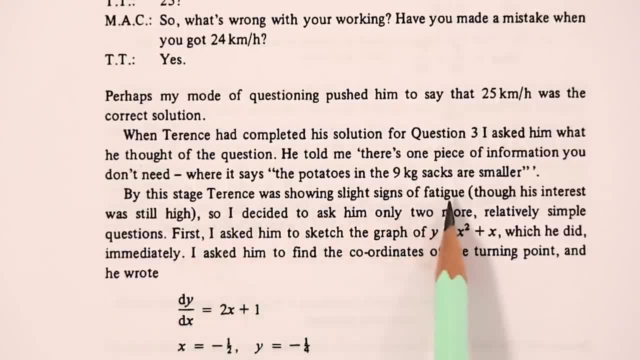 that at this stage Terence was showing slight signs of fatigue, although his interest was still high, So he asked him just two more relatively simple questions. First, he asked him to sketch the graph of y equals x squared plus x, which he did immediately. 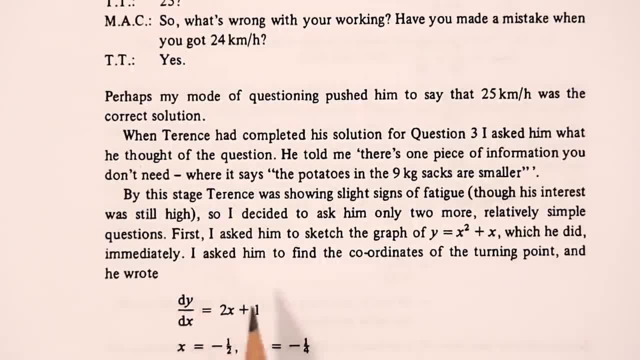 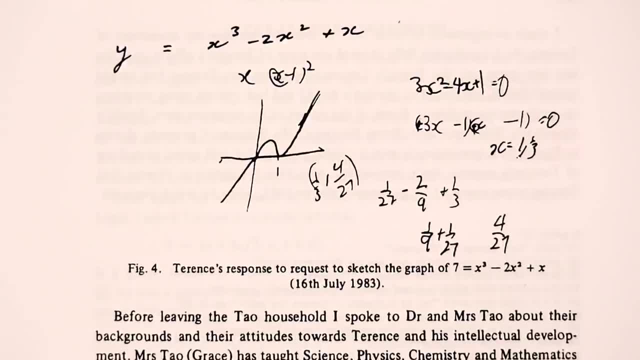 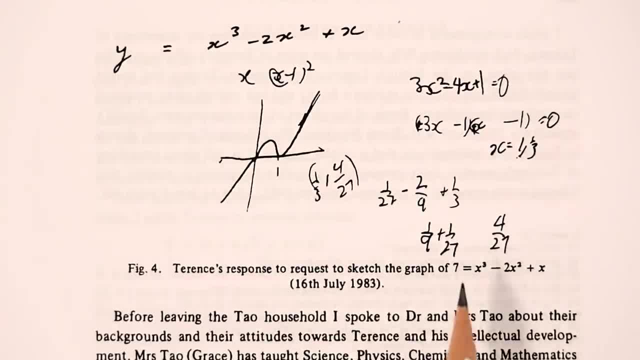 plus x, And in about one minute he produced this. It is interesting to note that Terence hadn't begun to study any calculus at school But when Clements had arrived at the Tau household and was speaking with Terence's parents, Billy 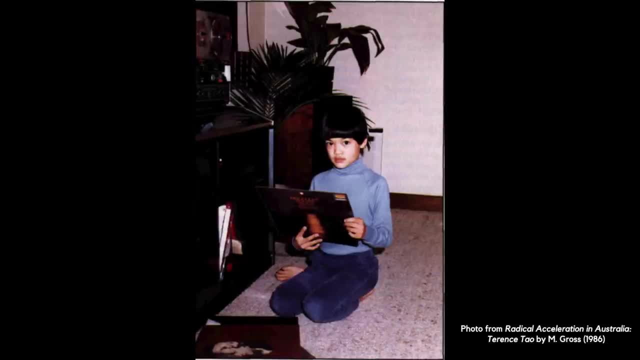 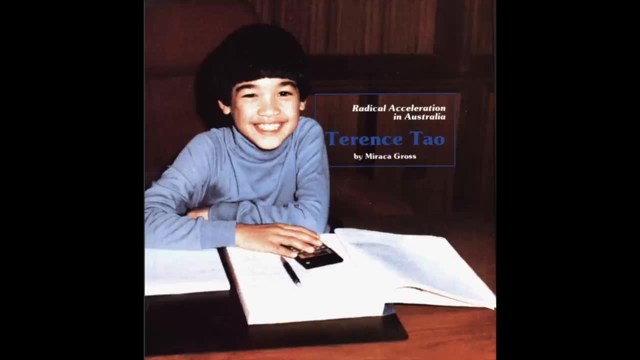 and Grace. he had spotted Terence sitting in the far corner of the room reading a book with the title calculus. Terence's dad was a doctor and Terence's mum was a graduate of physics and mathematics. He was a professor at the University of New York. 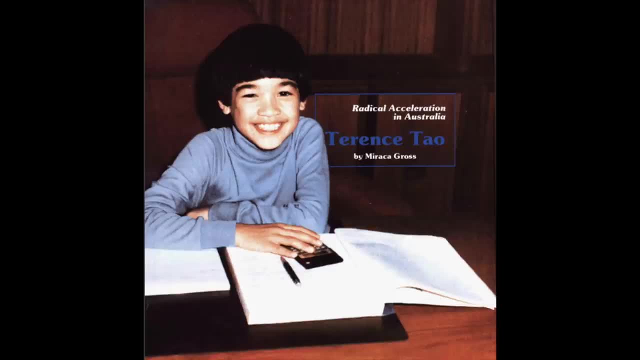 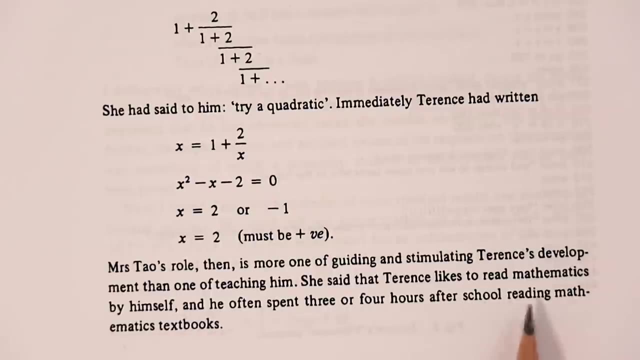 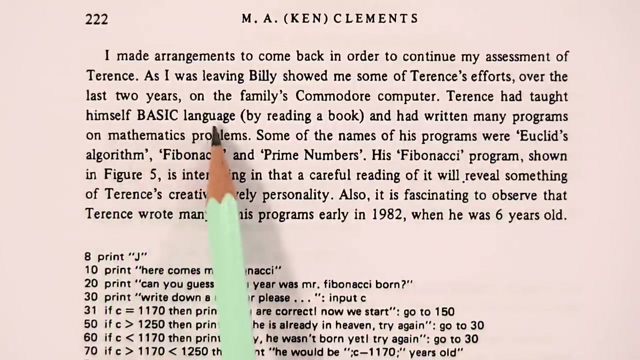 He had worked as a high school teacher. She said that Terence liked to read mathematics by himself and often spent three or four hours after school reading mathematics textbooks. Terence also had an interest in computer programming and had taught himself basic language by reading. 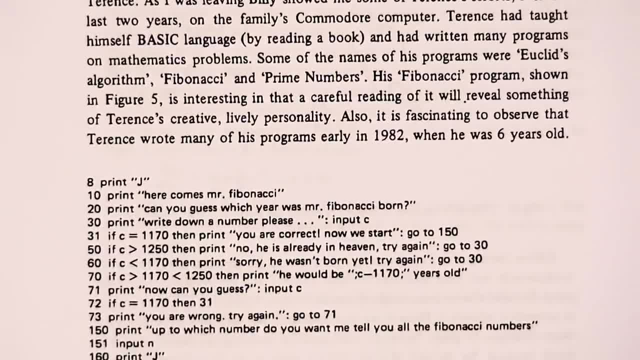 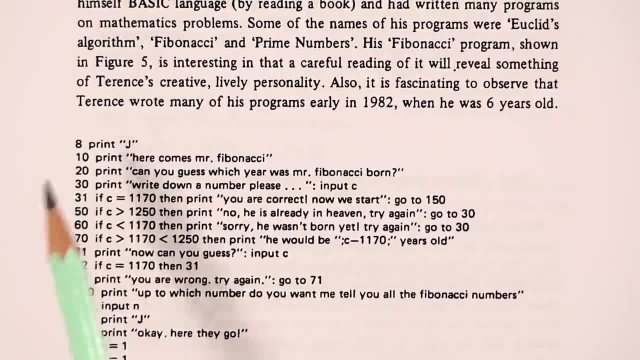 a book And at the end of this first visit, Clements was shown one of Terence's programs. It was called Fibonacci and actually contains plenty of humor. Apparently, Terence's father was a mathematician. Apparently, Terence wrote many of his programs when he was just six years old. 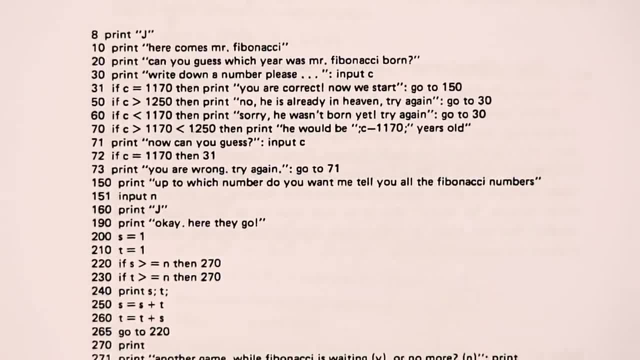 So let's take a look at Fibonacci. It doesn't just calculate the sequence It starts with. here comes Mr Fibonacci. Can you guess which year was Mr Fibonacci born? Write down a number, please. Then, if the user inputs the correct answer, they can start. 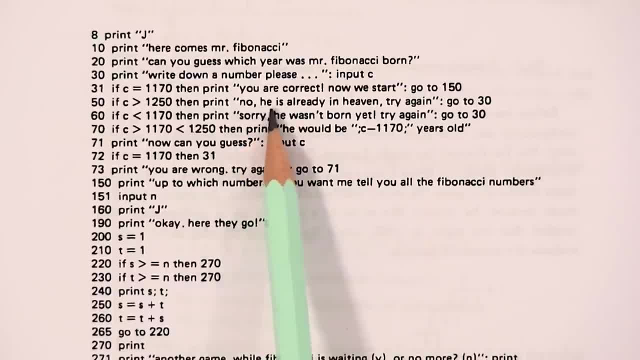 However, if their guess is too far off, they'll be told: no, he is already in heaven, Try again. Or they might be told: sorry, he wasn't born yet, Try again. Then, if they were close, it would print the difference between the guess and the actual. 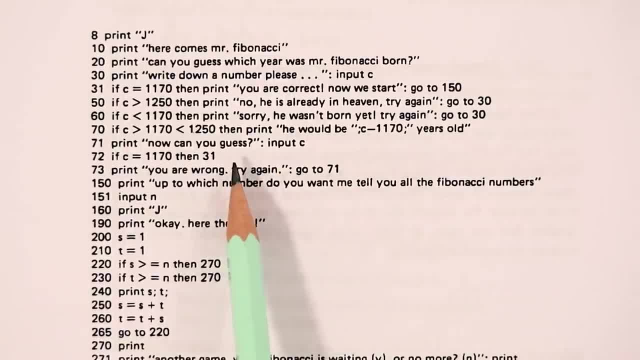 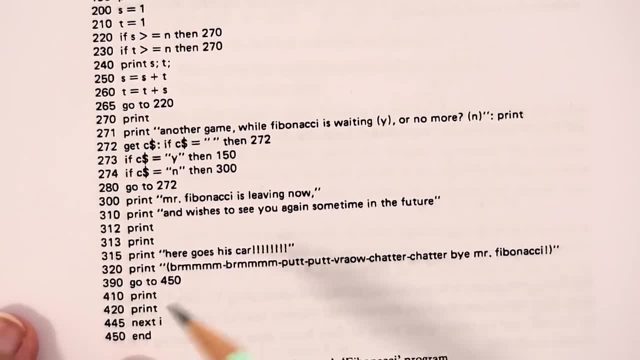 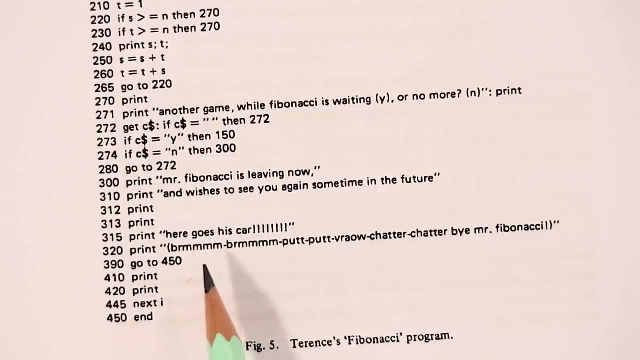 answer meaning that even to start this program, the user is guided by a bit of mathematics After printing some of the sequence it ends with: Mr Fibonacci is leaving now and here goes his car. This line is perhaps the only reminder of just how young the author of this program. 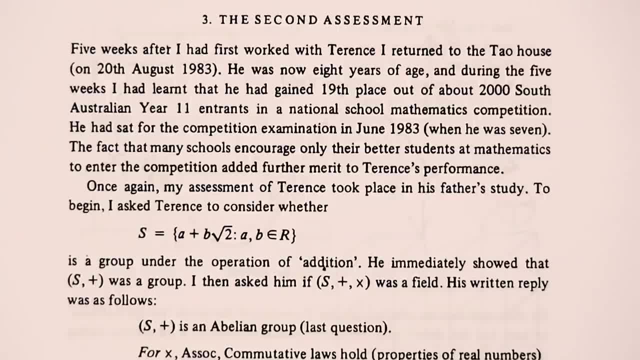 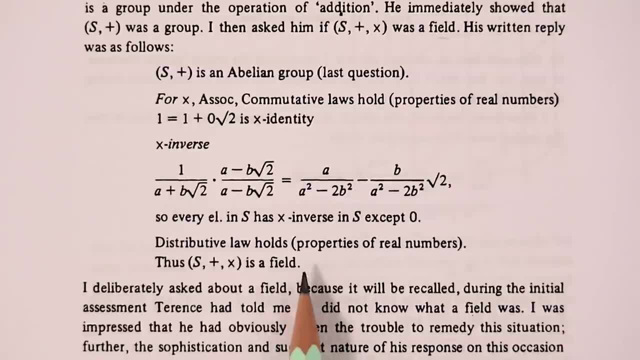 is Five weeks later. Clements came back for a second visit and he asked Terence if something was a field. Here was Terence's answer, clearly demonstrating that since the last visit he now knew exactly what a field was. This kind of answer is something that a university student would be proud of, and it shows just 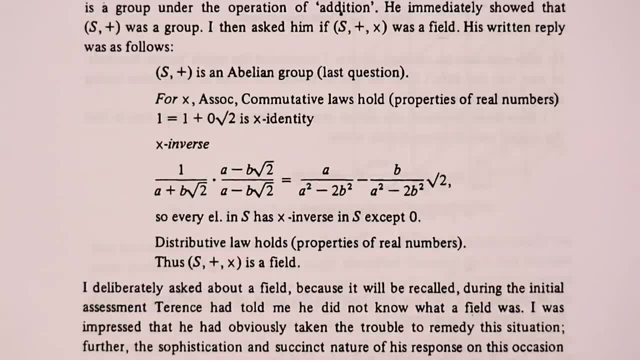 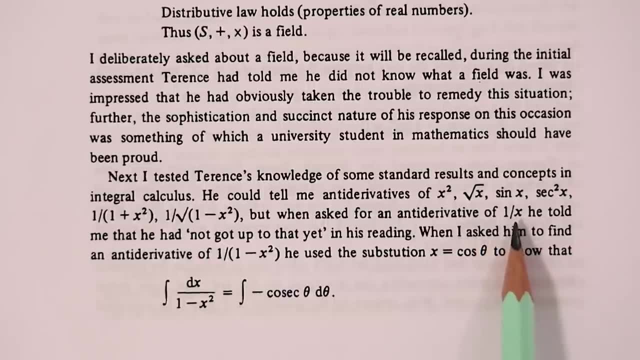 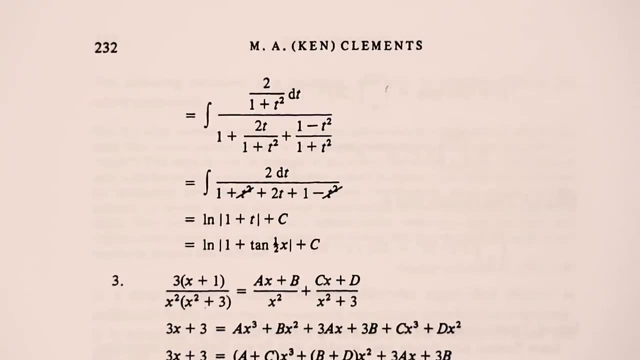 how fast Terence was able to learn concepts. They encountered another thing, though, that he didn't know yet. he was asked for the antiderivative of one over x and responded that he had not got up to that yet in his reading. But on a third visit, not long after the second, Terence had not only mastered the antiderivative, 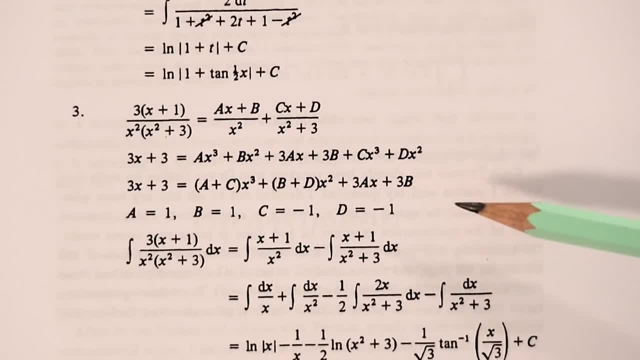 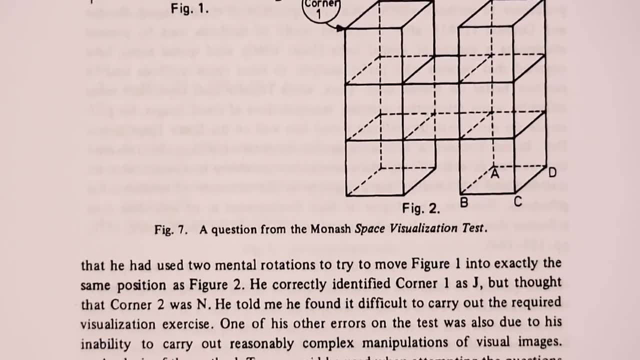 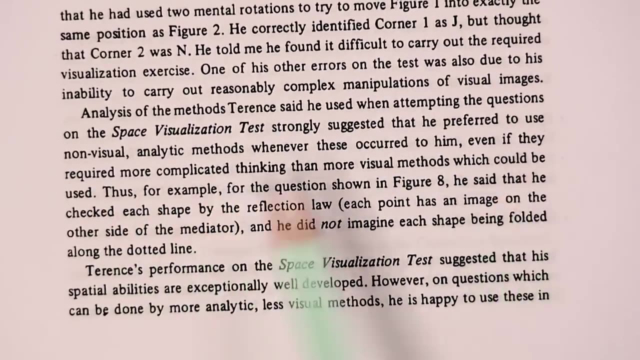 of one over x, but was doing things like this with partial fractions. He was given a space visualization test, which again made Clements come to the conclusion that Terence preferred to use non-visual analytic methods. Even if he was able to do that, he didn't know how to do it. 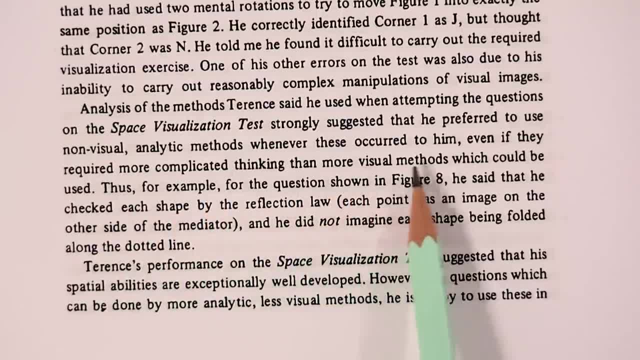 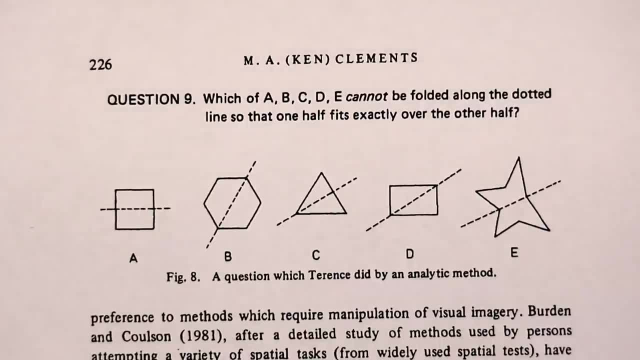 Even if they required more complicated thinking than more visual methods. For example, with this question here, Terence said that he checked each shape by the reflection law, which was that each point had an image on the other side of the mediator, and he 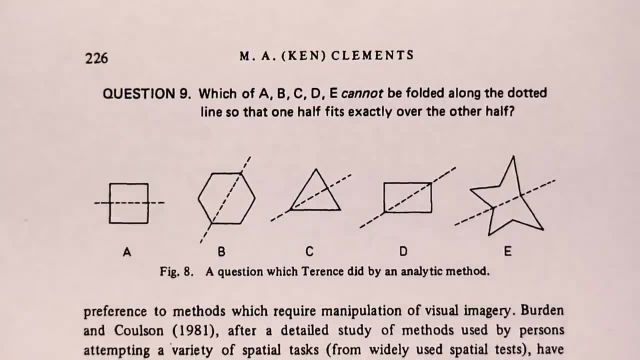 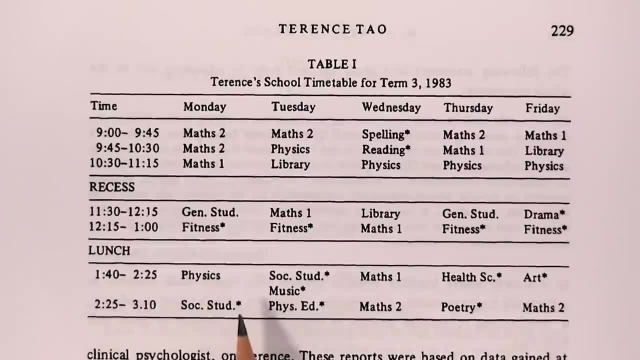 did not imagine each shape being folded along the dotted line. Included in the report was Terence's school timetable. The subjects marked with the asterisk took place at the primary school, While the subject was not marked with the asterisk. the subject was marked with the. 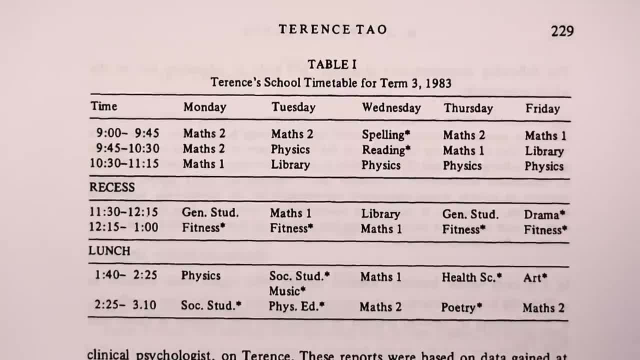 bazaar, While all the others took place at the high school. His teachers said that, whilst 7 year old Terence did have the academic ability of a 16 year old, his maturity was still that of a 7 year old, And Terence's parents had to balance giving him a childhood that challenged him intellectually. 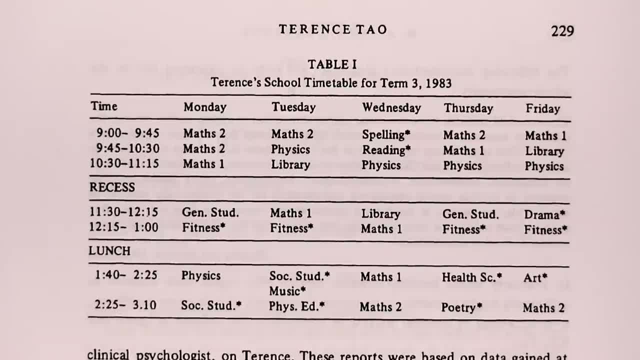 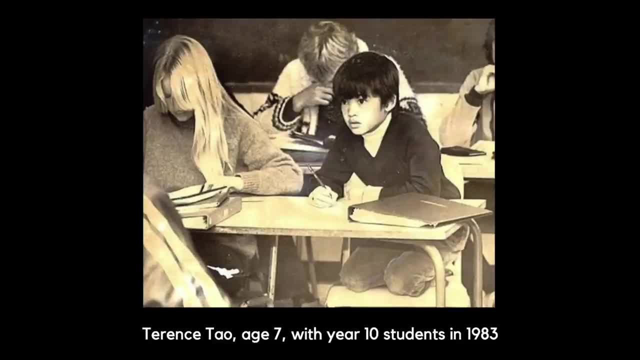 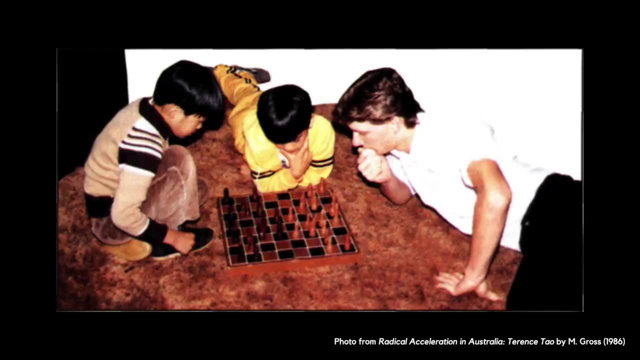 but also allowed him to fit in socially and emotionally. The report makes it clear that, rather than being pushed along one rigid track of mathematical, Terence was allowed to pursue the topics that interested and challenged him the most. He loved mathematics, and the efforts of those around him were to 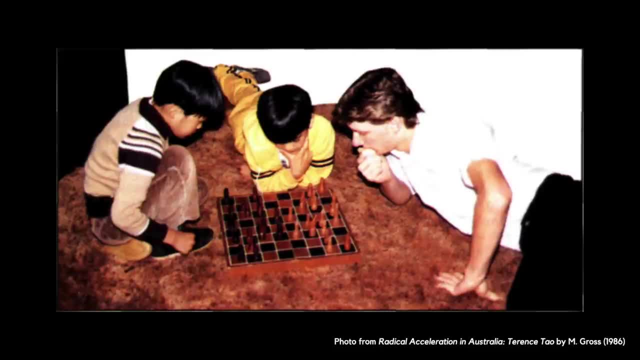 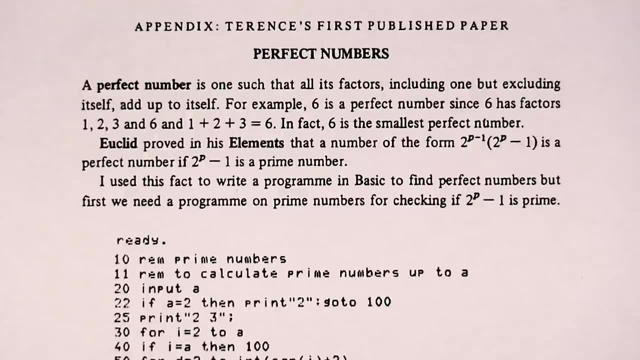 ensure that he did not become bored or frustrated with non-challenging work. Let's finish with a look at a program that now eight-year-old Terence Tao had submitted for publication to a student mathematics journal called Trigon. It is all about perfect numbers and is labeled here as Terence's first published paper. 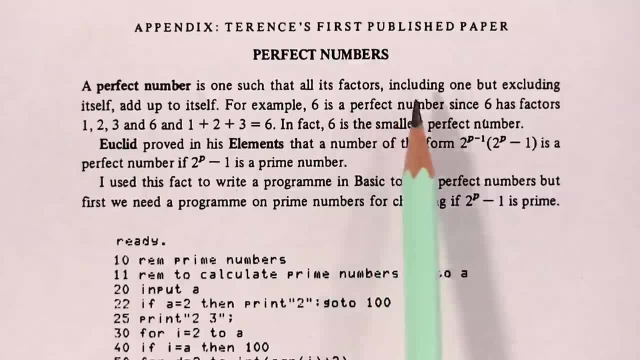 A perfect number is one such that all its factors, including one but excluding itself, add up to itself. For example, 6 is a perfect number because 6 has factors 1, 2, 3 and 6, and 1 plus 2 plus 3 is equal to 6. Euclid proved that a number of this 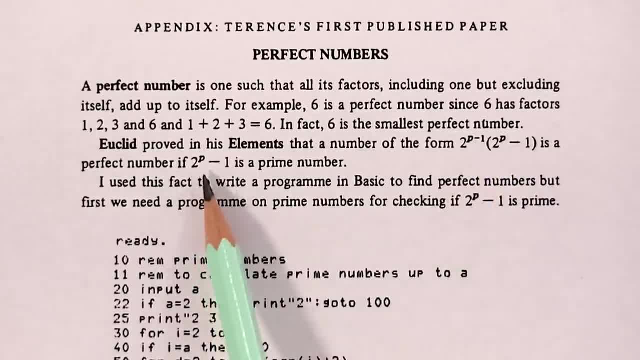 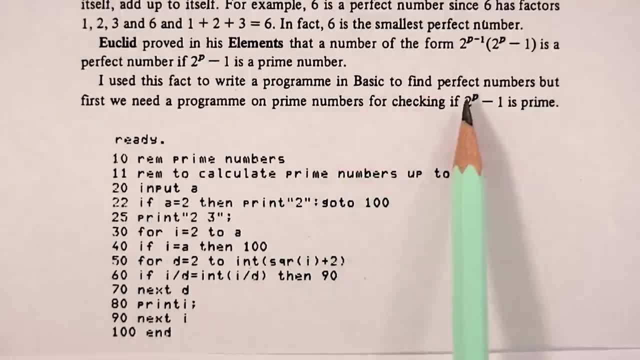 form is a perfect number. if 2 to the p minus 1 is a prime number. so Terence says that he has used this fact to write a program in basic to find perfect numbers, which starts with a program for checking if 2 to the p minus. 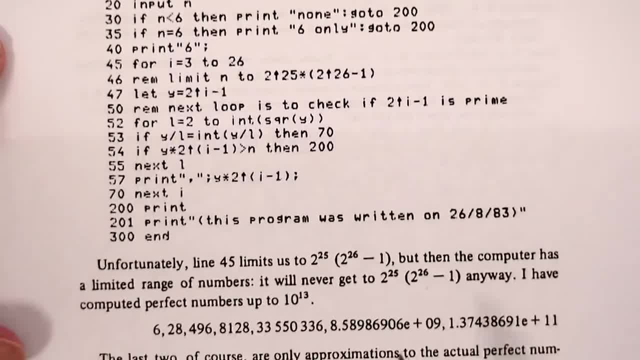 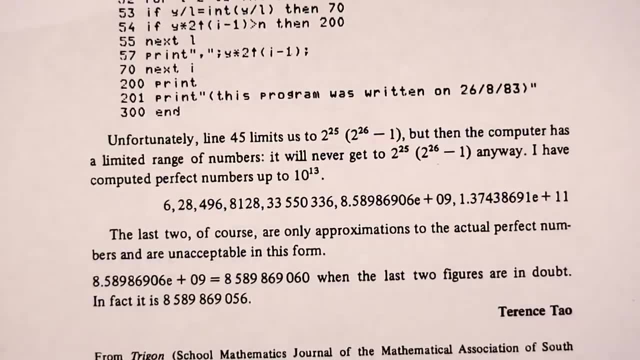 1 is prime. Then he computes perfect numbers up to 10 to the 13.. Yet again, another example of just how outstanding he is. It's been humbling for me to read through these notes. I hope that it doesn't seem discouraging to any. 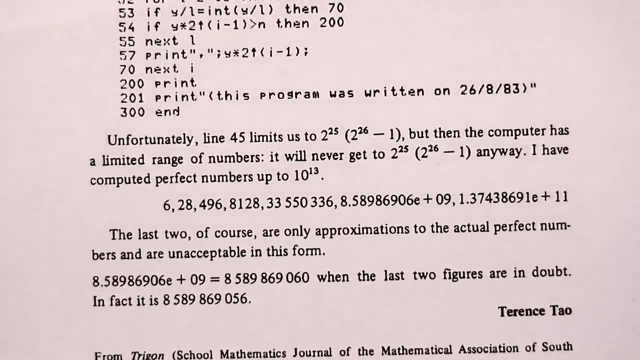 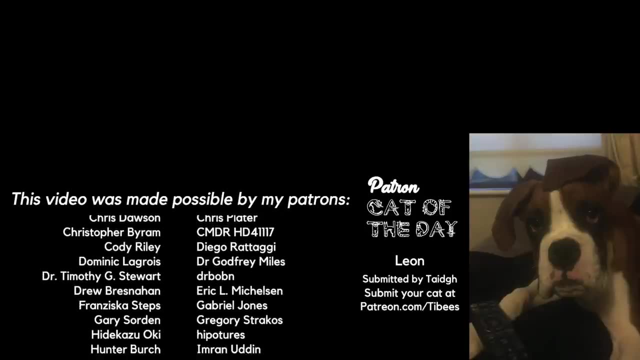 aspiring mathematician out there, as I'm sure Terence Tao would even agree that many of the great mathematicians followed a more conventional path through education. Thanks for watching. I hope you've enjoyed this video and thanks, as always, to my Patreon supporters for making these videos possible. A special shout. 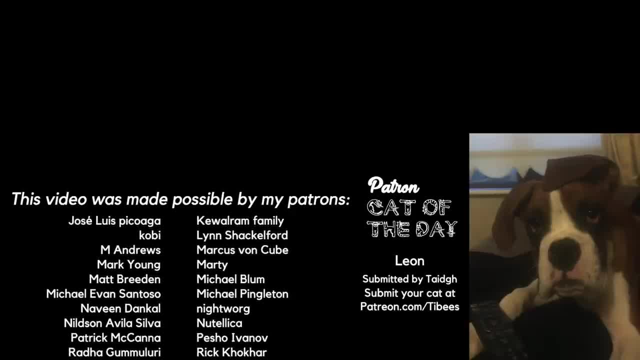 out to today's Patreon cat of the day, Leon.